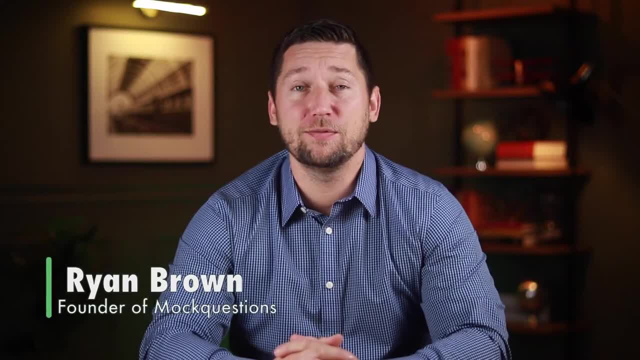 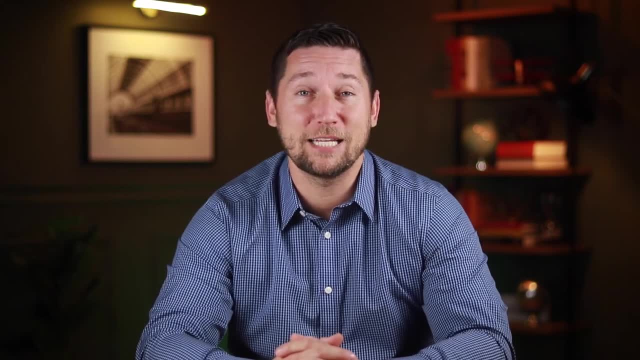 Hi, this is Ryan Brown from MockQuestionscom. In this video we'll discuss five environmental engineer interview questions from our website. We'll go over each question and some advice on how to answer them, along with an answer example Afterwards. if you found this video helpful, 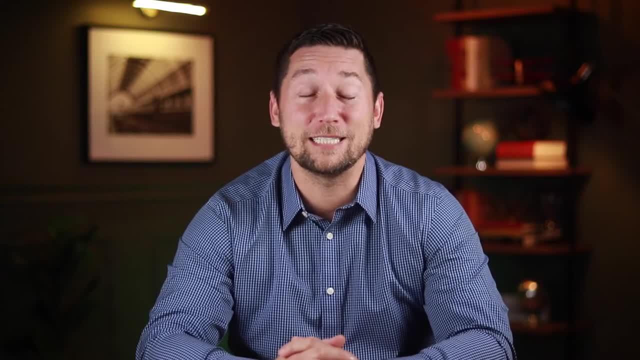 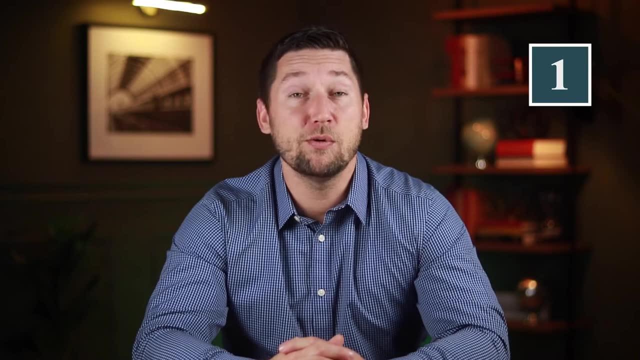 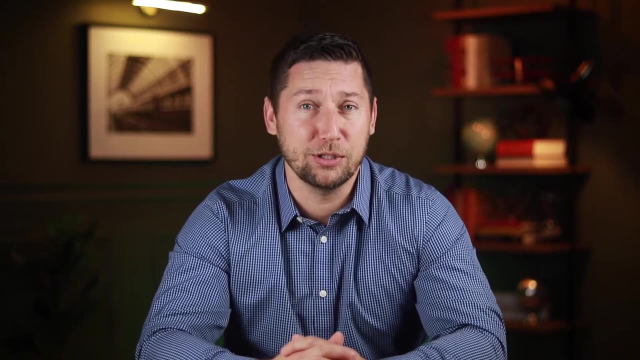 please like and share. That would mean a lot to us. Okay, let's get started. Question number one: If you are hired, what is the first contribution you will make to this company? Often in job interviews you will get a question about how you will contribute or add value to a 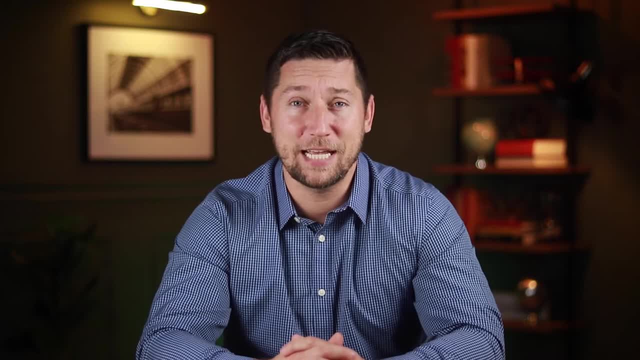 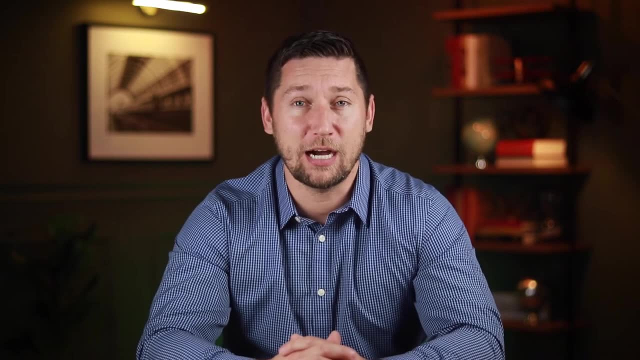 company. This question gives you a chance to explain what makes you stand out from other candidates and how you will be an asset to the company. The best way to answer it is to give examples of what you have accomplished in the past and relate them to what you can achieve in the. 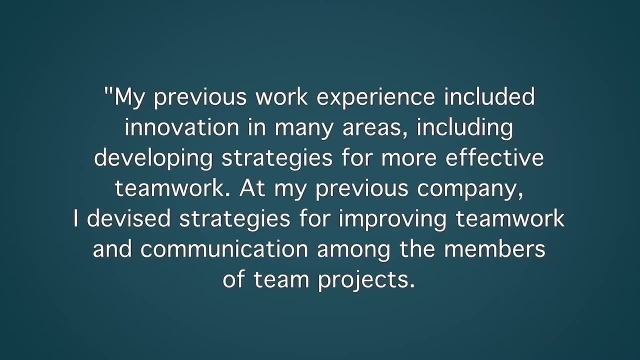 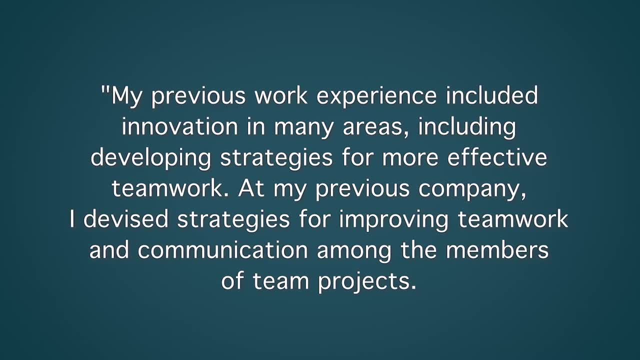 future. Here is our answer example: My previous work experience included innovation in many areas, including developing strategies for more effective teamwork. At my previous company, I worked as a sales manager for a company that was in the sales department. I worked as a sales. 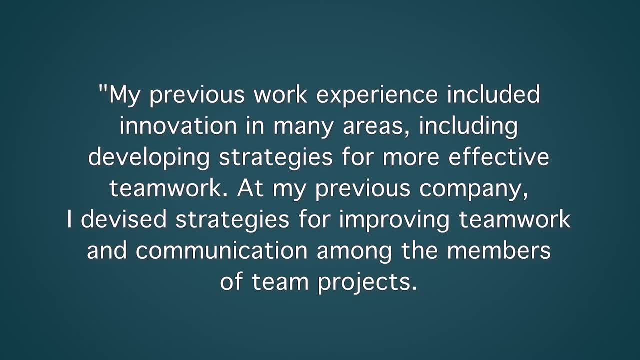 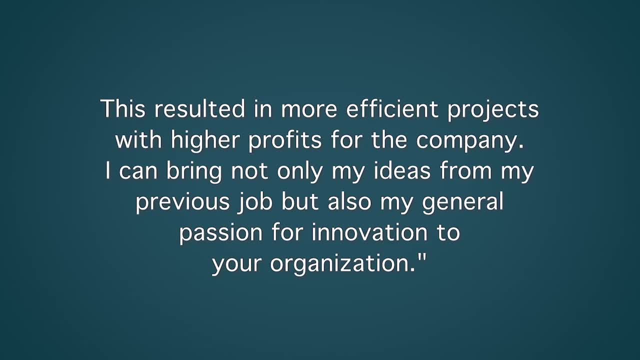 manager for a company that was in the sales department. I devised strategies for improving teamwork and communication among the members of team projects. This resulted in more efficient projects with higher profits for the company. I can bring not only my ideas from my previous job. 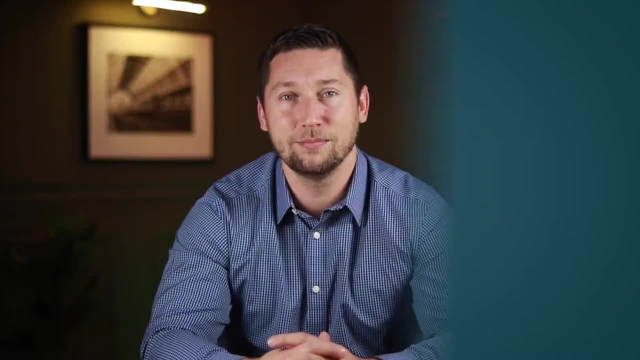 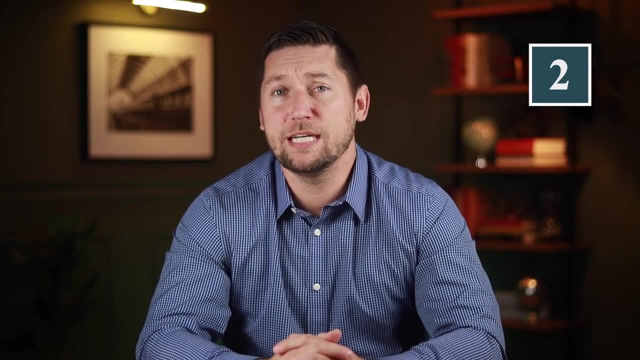 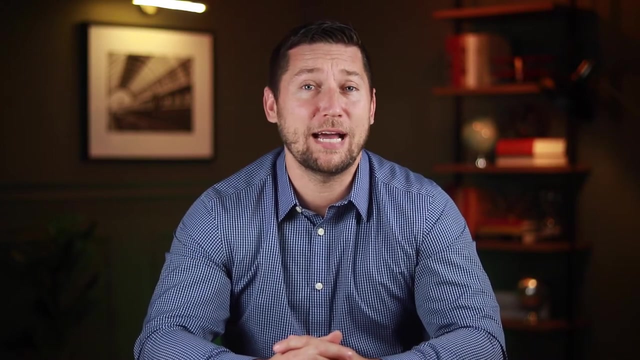 but also my general passion for innovation to your organization. Question number two: What advice would you offer someone considering a career in environmental engineering? The interviewer is asking this question to hear more about how you got into environmental engineering and what you like most about it. They want to know. 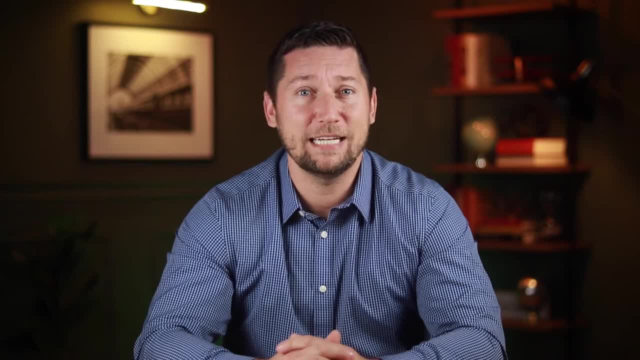 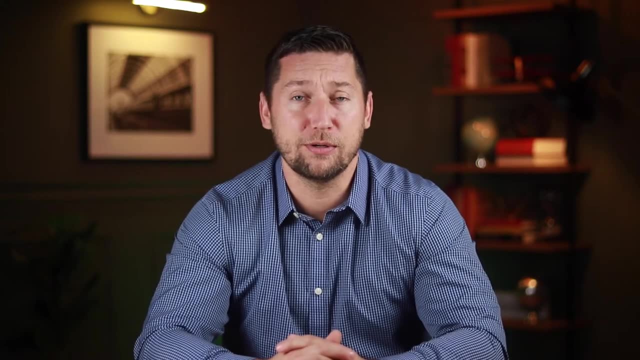 more about what aspects of the profession you are most passionate about and if that fits with their company's goals and vision. You can discuss how a professor or relative inspired you to pursue the career, or discuss your strong interest in protecting the health, welfare and security. 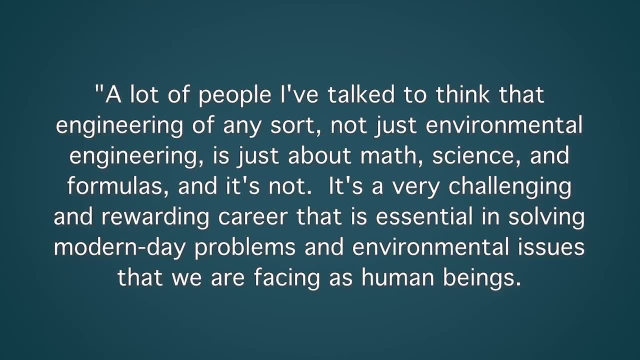 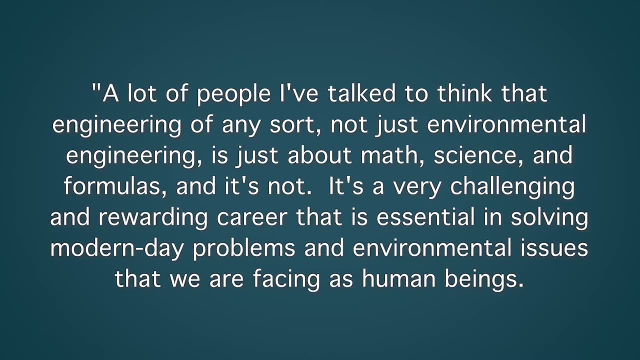 of future generations. A lot of people I've talked to think that engineering of any sort, not just environmental engineering, is just about math, science and formulas, and it's not. It's a very challenging and rewarding career that is essential in solving modern day problems. 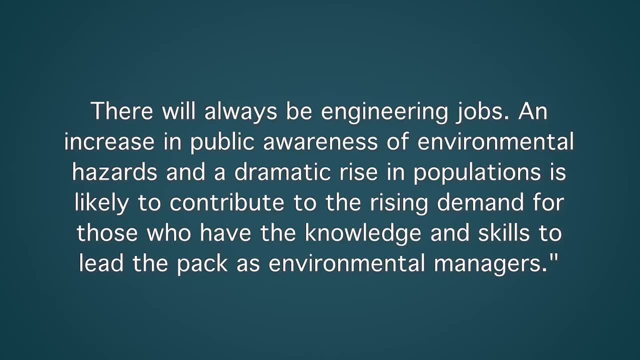 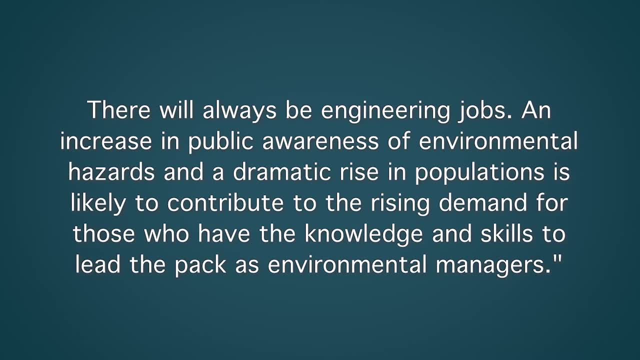 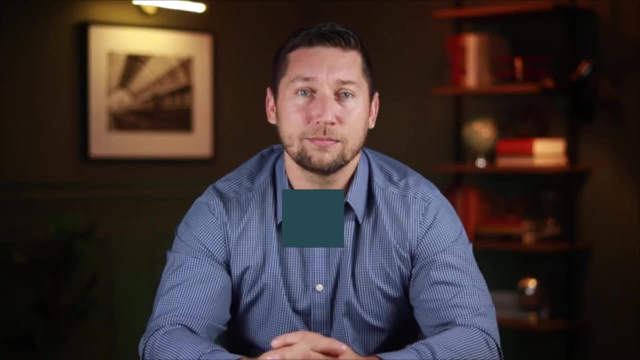 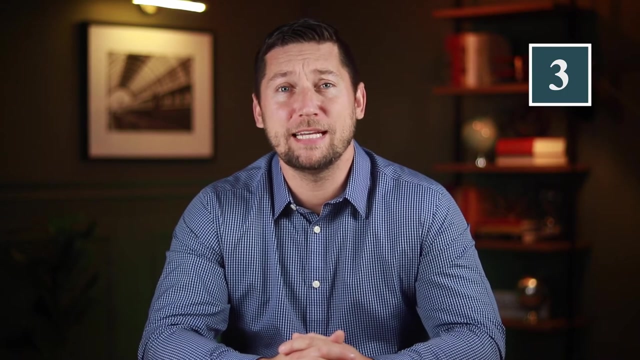 and environmental issues that we are facing as human beings. There will always be engineering jobs. an increase in public awareness of environmental hazards and a dramatic rise in population is likely to contribute to the rising demand for those who have the knowledge and skills to lead the pack as environmental managers. Question number three: How do you explain? 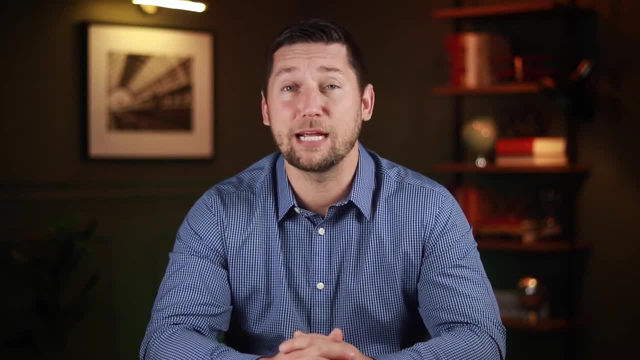 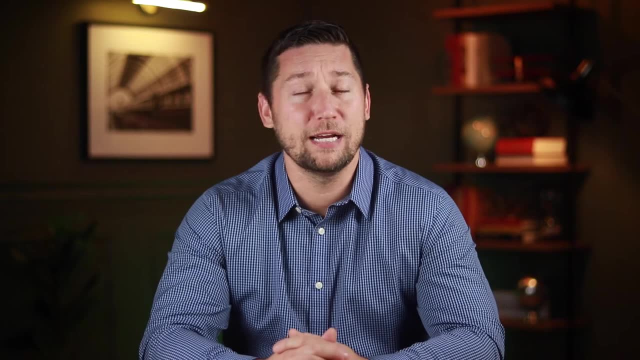 engineering concepts. There are a number of ways to explain engineering concepts. One way to explain engineering concepts is to list some engineering ideas to an audience who's unfamiliar with the topic during a presentation or an important meeting. An environmental engineer will work with many different people. It's essential to let your interviewer know that. 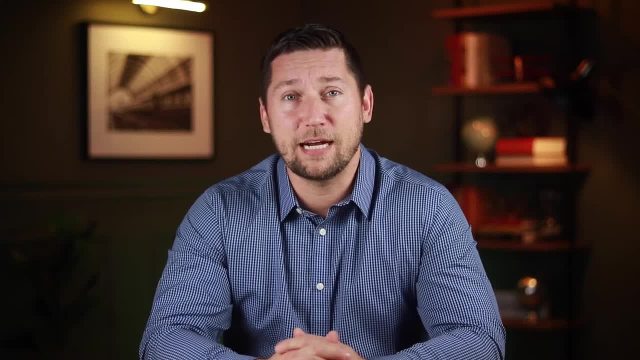 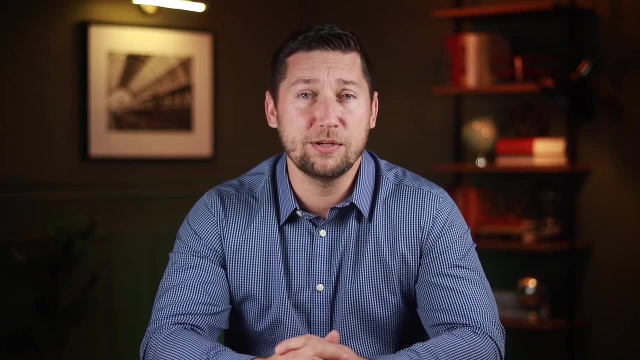 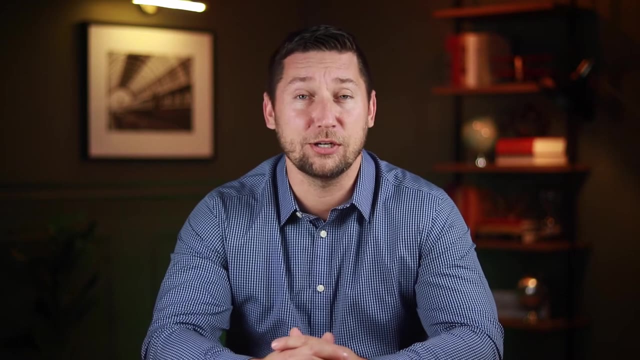 you are confident in communicating complex engineering topics to people of any skill level and background. Your answer should clarify that you have a strong understanding of engineering concepts and understand the importance of communicating those concepts Before the interview, how to simplify them so that others can understand the big idea in terms they can relate to. 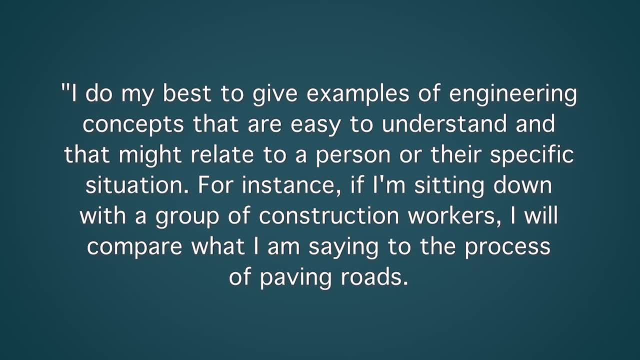 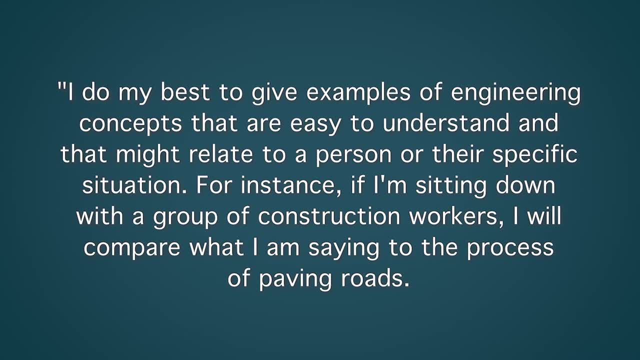 I do my best to give examples of engineering concepts that are easy to understand and that might relate to a person or their specific situation. For instance, if I'm sitting down with a group of construction workers, I will compare what I am saying to the 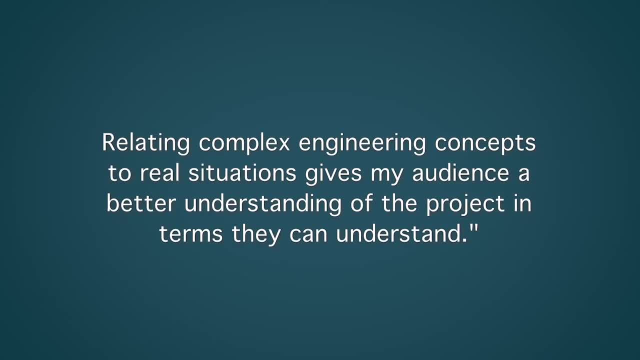 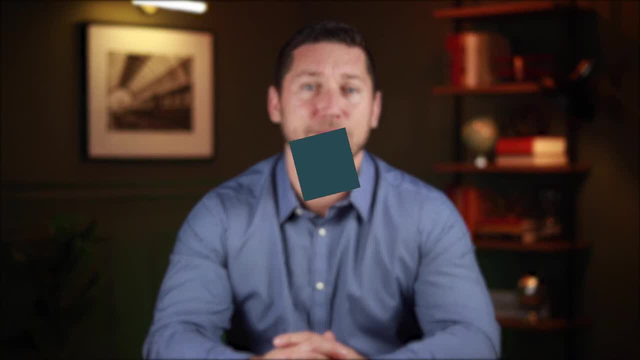 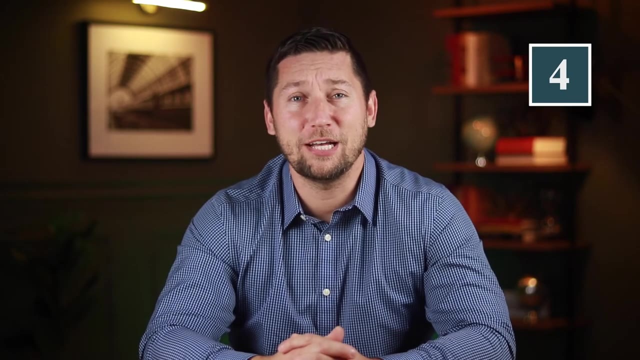 process of paving roads. Relating complex engineering concepts to real situations gives my audience a better understanding of the project in terms they can understand What's a real challenge. If you fit in a position where you're almost impossible to cheat, want to break or fail in a position, you should choose a job. 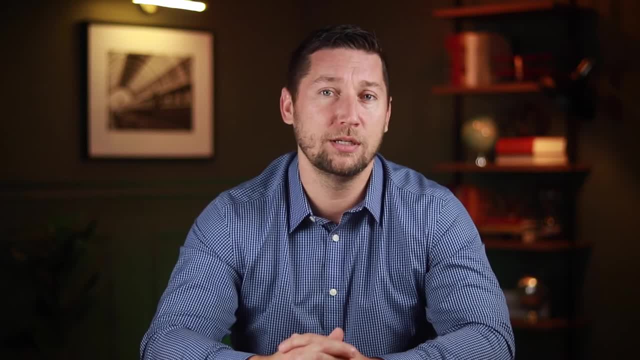 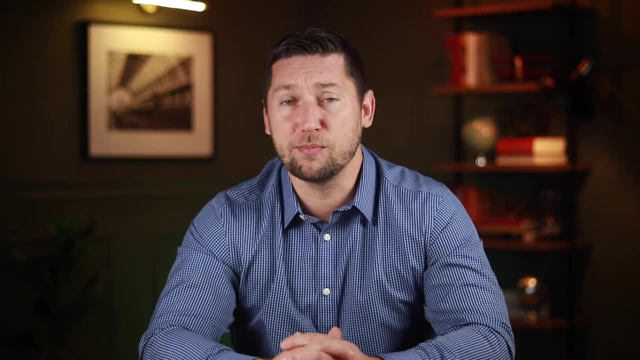 Question number 4,. what will be your biggest challenge in this position? In an interview, the employer's ultimate goal is to assess if you are a good fit for the position. To do this, the interviewer may have you reflect on what you think are the most challenging aspects. 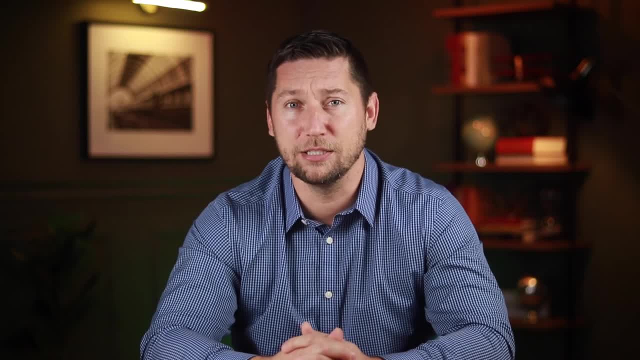 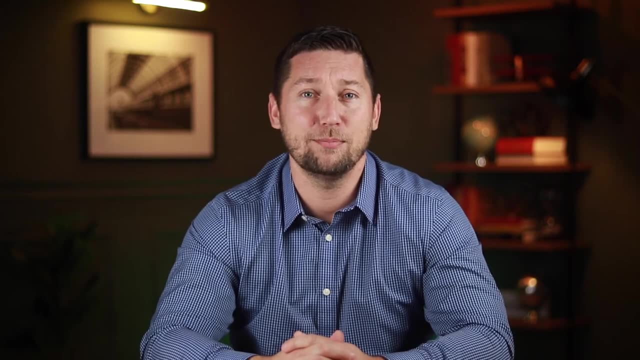 components and thinking about what you need in terms of skills and knowledge to accomplish each task. Think about any elements of the job that will require training or additional time to learn, and be honest in your response. You can also mention that you are motivated by challenges. 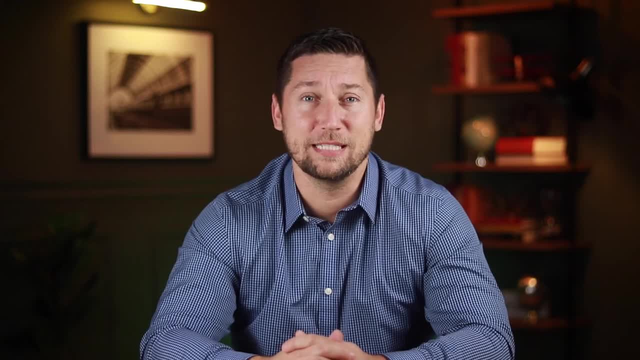 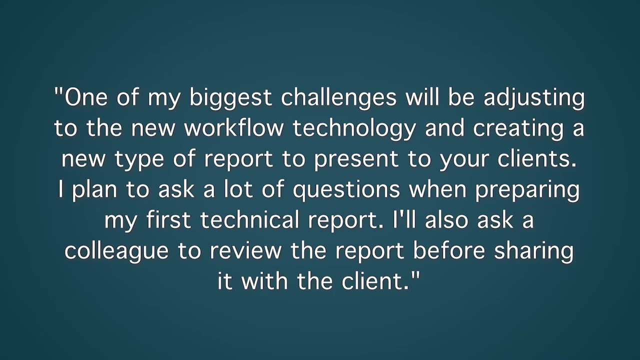 can effectively meet challenges and have the flexibility and skills necessary to handle a challenging job. One of my biggest challenges will be adjusting to the new workflow technology and creating a new type of report to present to your clients. I plan to ask a lot of questions.